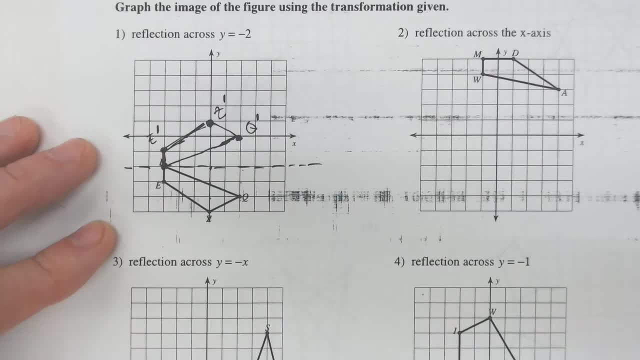 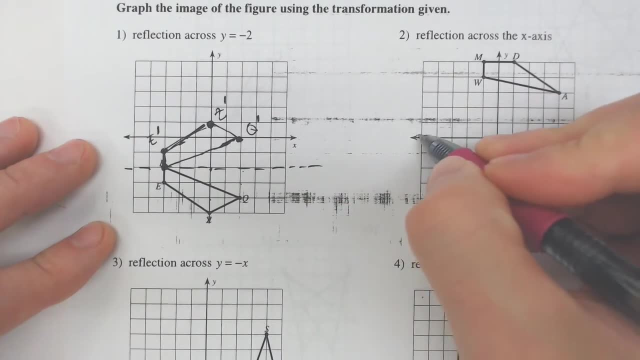 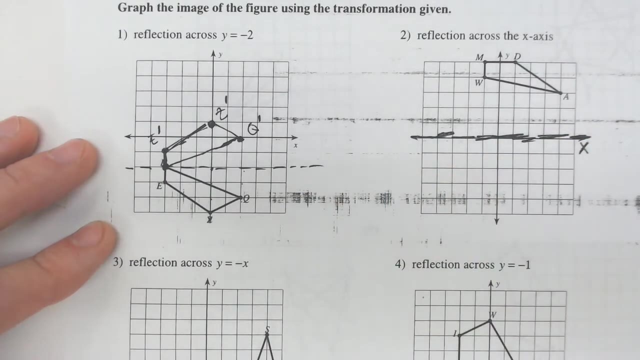 The next problem is going to reflect across the x axis. The x axis is this one right here. So I'm going to put a big dotted line here, as aggressive as I can make it, so we can see it. And then we just count: how far do we go down? Go down by that same amount. We went down by 1, 2, 3 from point a. so I go down by 1, 2, 3 and I label it a prime. 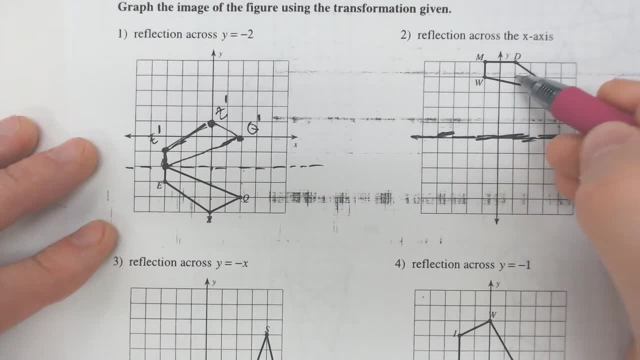 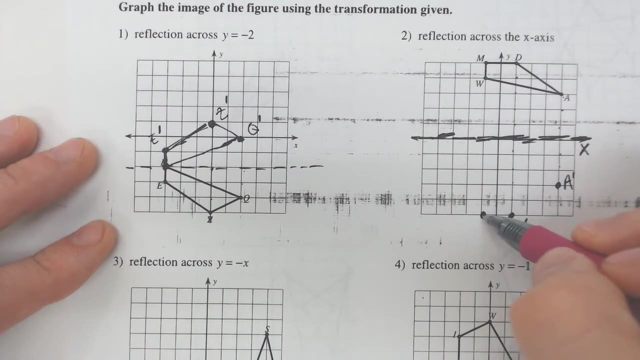 For point d: we went down by 1, 2, 3, 4, 5.. I go down by 1, 2, 3, 4, 5 and I label it d prime. Point m: I went down by 5.. I go down by 5 more. Point w: I went down by 4.. I go down by 4 more And I connect the dots by tracing it out and I should have the same shape that we did last time. 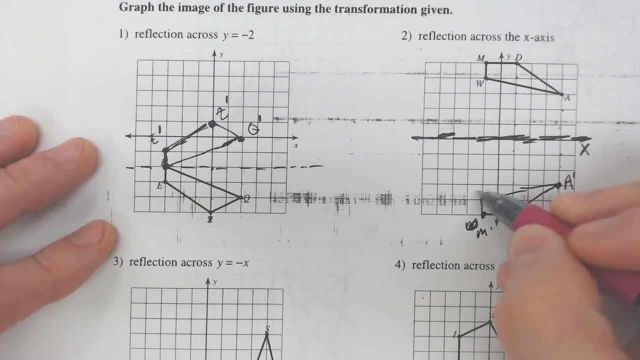 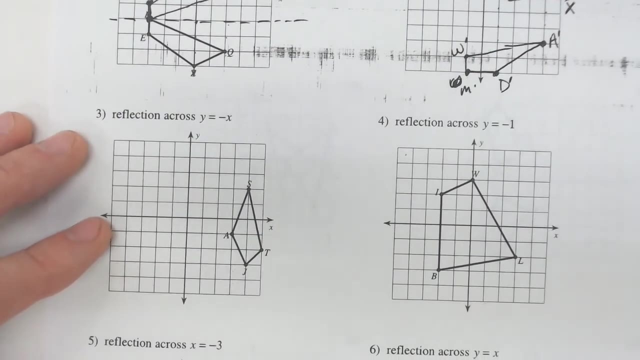 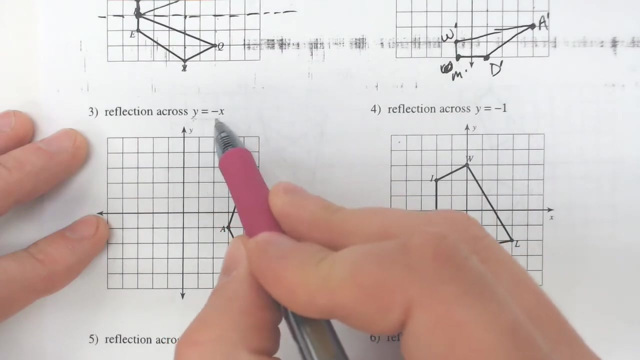 Make sure we label it m prime, w prime and d prime. Now, the next two are going to be a little bit different because they're going to be reflecting across. Well, the next one is going to be a little bit different. It's going to be reflecting across. y equals negative x. 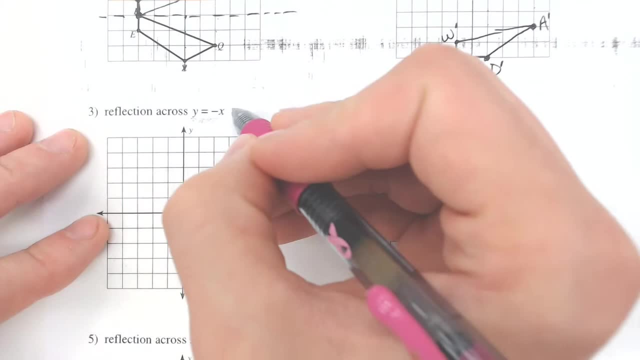 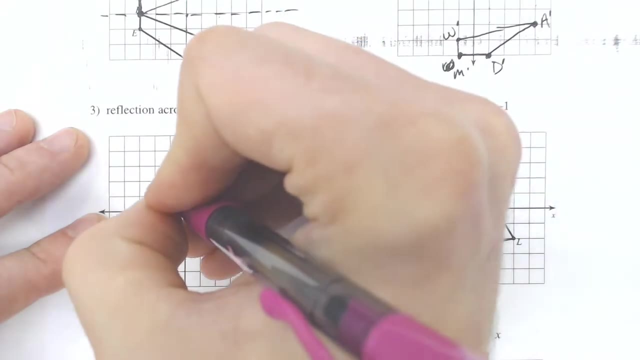 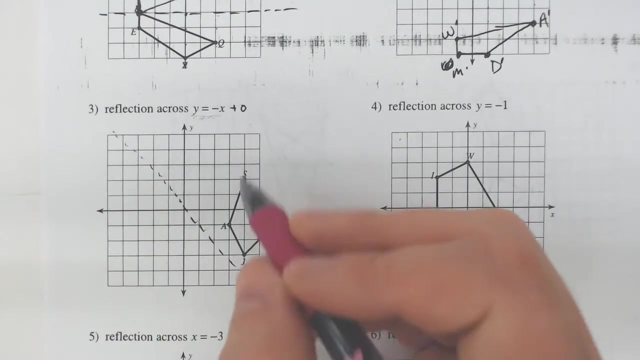 So y equals negative, x has a slope of 1 and a y intercept of 0. So y equals negative, x has a slope of 1 and a y intercept of 0.. If I drew that line right here, our shape is going to need to flip over that, which is going to be a little bit more difficult because it's not going to be just straight up or down or left and right. 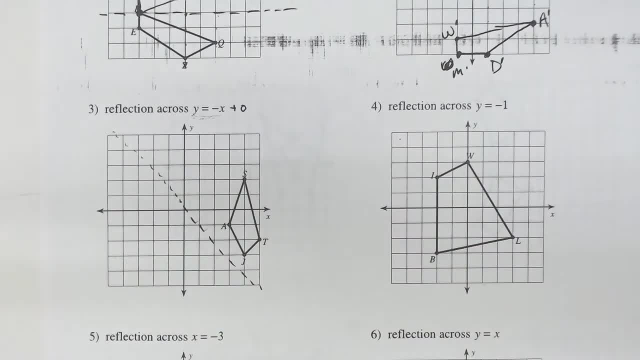 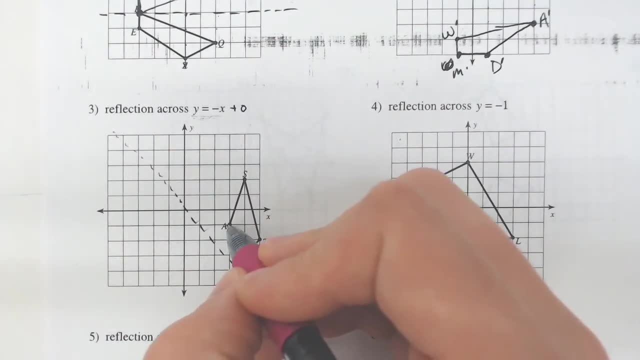 It's going to be a diagonal distance and sometimes the diagonal just doesn't work. So if you have this situation, you might be able to count the diagonal distance and be like, oh, we went a diagonal distance of 1.. We can go a diagonal distance of 1 more. 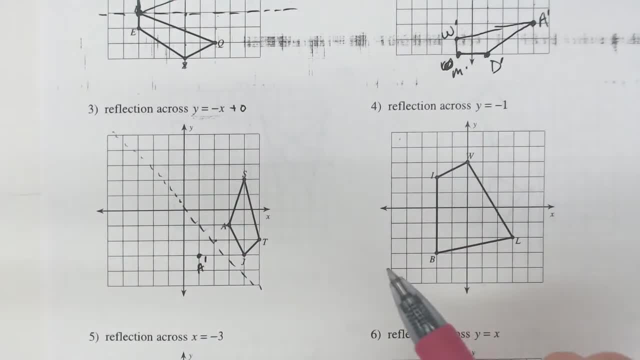 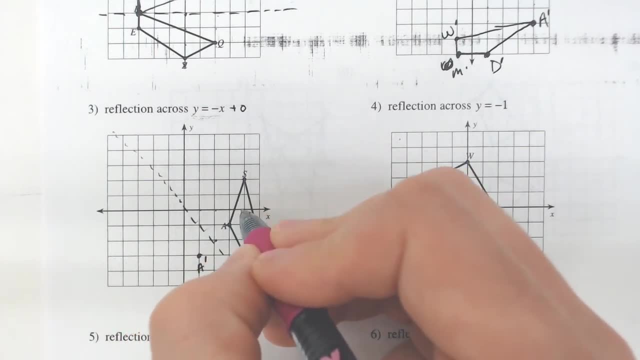 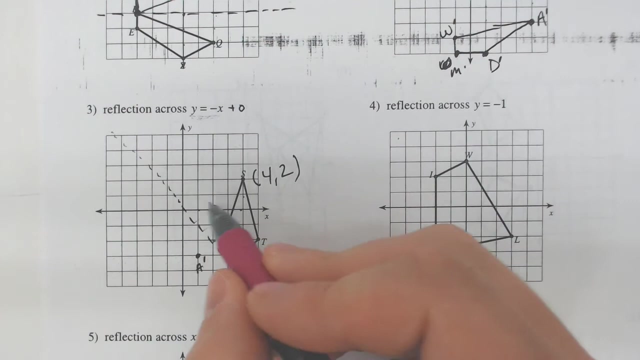 But occasionally that's going to be really difficult to do. So what I would like you to do is label these points literally by what they are: 1, 2,, 3, 4, comma. 2 is point S, And point A we already did was 1, 2, 3, comma, negative 1.. 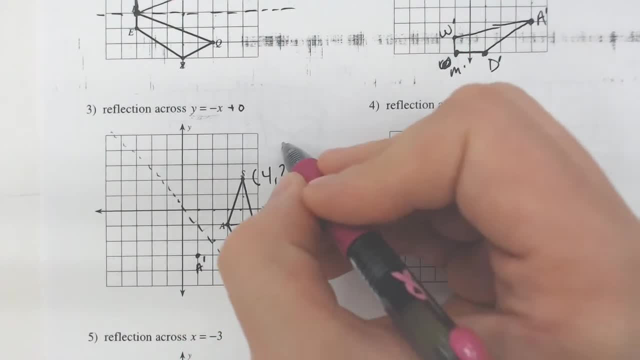 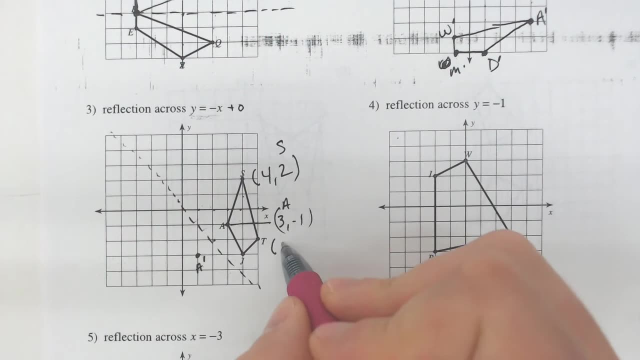 3, comma, negative: 1. A, Point T is at 1.. 2,, 3,, 4,, 5, comma, 2, negative: 2. And point J is at 4,, negative: 1,, 2, 3.. 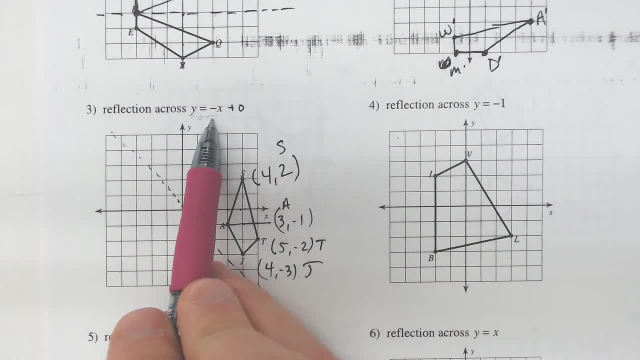 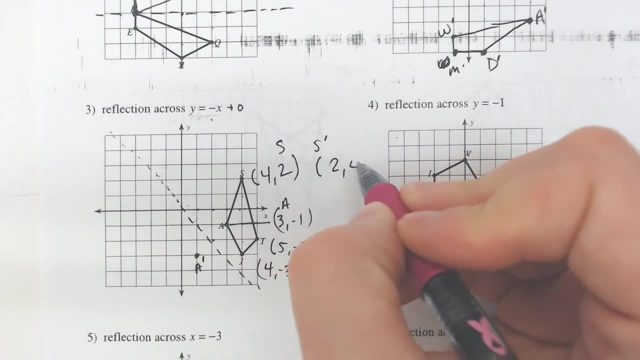 If it is reflected across y equals x, we will end up switching the signs. So my S prime is going to be the flipping of these. 2, comma 4.. That's, if you're reflecting across y equals x, But this is not just y equals x, this is y equals negative x. 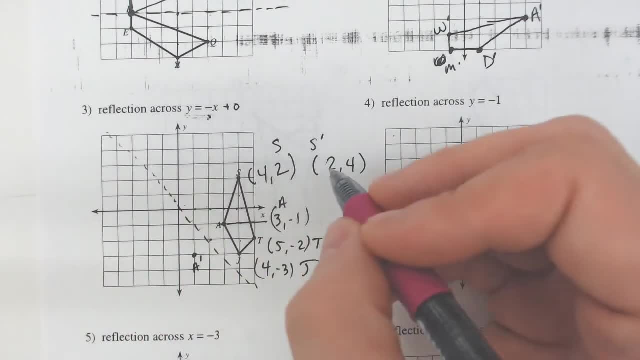 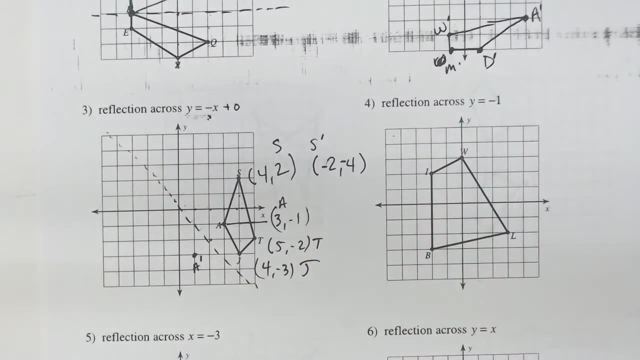 So, because it's y equals negative x, I'm not just going to switch these, I am also going to switch the signs of both of them. So you switch the x and y and you switch the signs when you're reflecting across: y equals negative x. 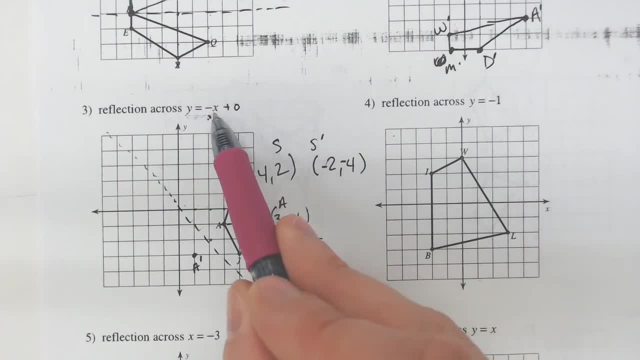 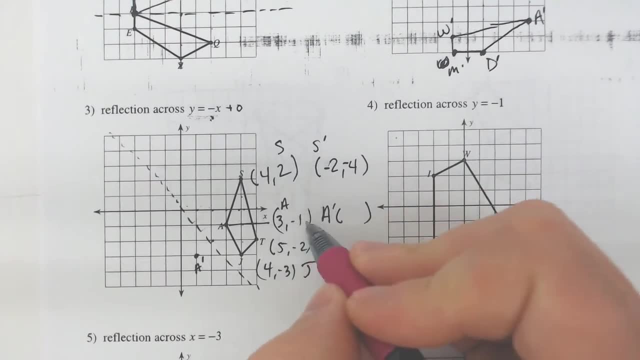 Y equals regular x. we just switch the x and y. So for my A prime, I'm going to switch these 2, negative 1 and 2.. Negative 1 and 3. And because it's negative x, I am going to also switch the signs of both of them. 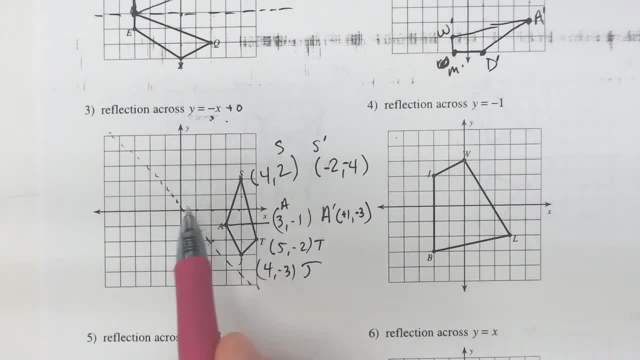 And let's see if I actually got it right, Because I counted diagonal. let's see if I got it right for my A prime. Is it at positive 1, negative 3? 1, 2, 3.. Yes, it is. 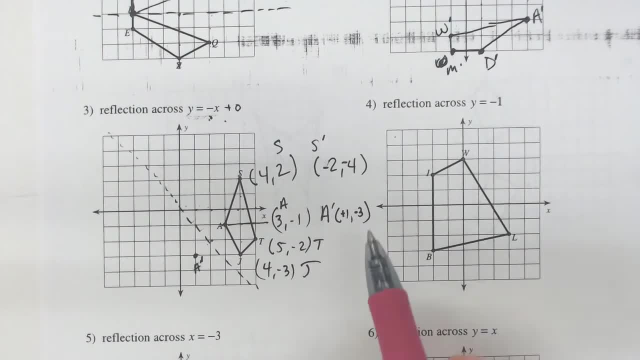 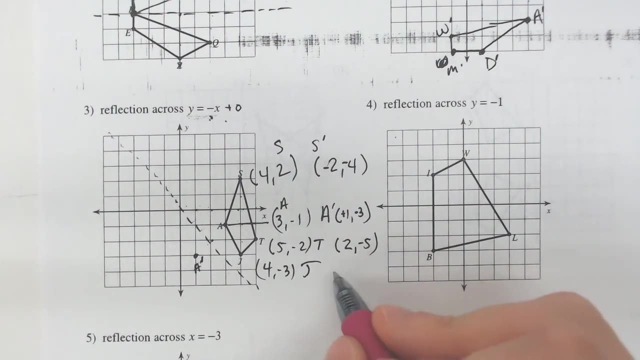 So my A prime I was able to do Switching my T would end up being positive, 2.. Positive, 2, negative, 5 when I switch both of them and switch the signs. And switching my J would end up being positive, 3, negative, 4 when I switch them and switch the signs. 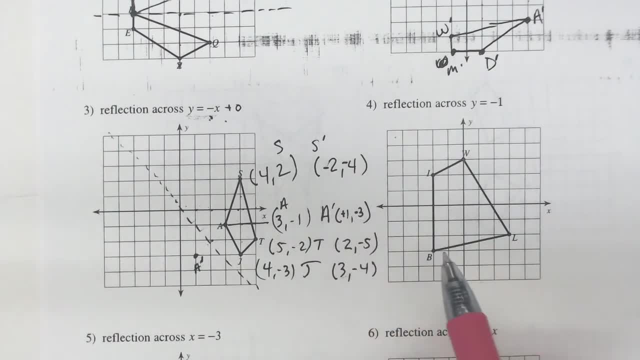 So I'm going to plot these points, except for A. I've already plotted point A, So I'm going to start with S, I'm going to go to the negative 2, then negative 1,, 2,, 3,, 4.. 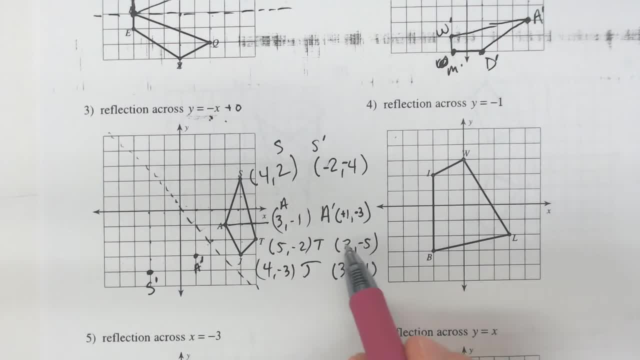 And label that S prime. Then I'm going to plot point T, which is at positive 2, negative 5.. I'm going to label that T prime Went to the right by 2, down by 5.. And then J prime is going to be 3, negative 4.. 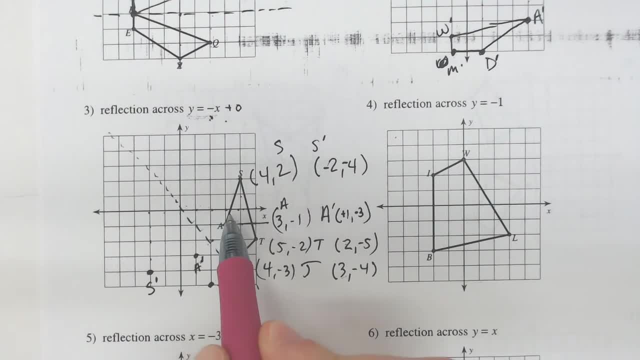 So I'm going to go to the right by 1,, 2,, 3.. And then down by 4.. 1,, 2,, 3,, 4.. For J prime: When I connect these dots It will: 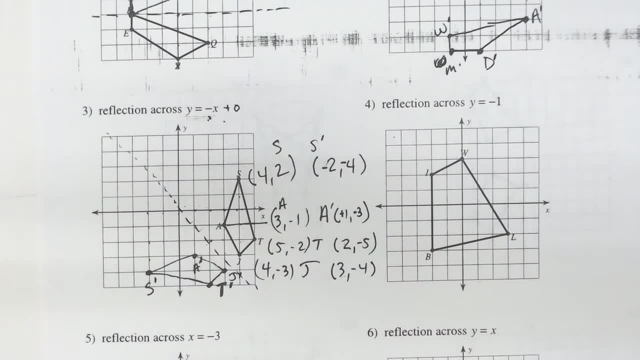 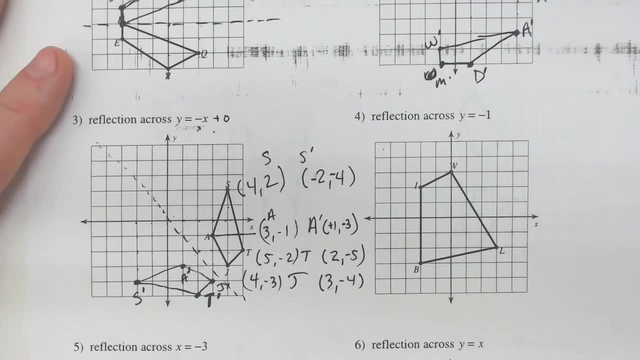 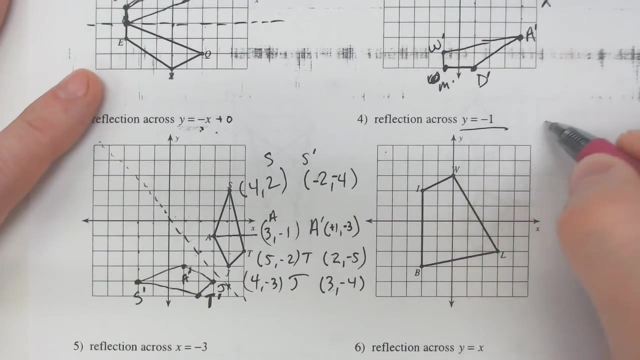 Give me that shape, that flipped over and folded over that dotted line. So we're going to try one more. We're going to reflect across Y equals negative 1. And that's going to be another horizontal line. Y equals is horizontal. If it is X equals, it's going to be vertical. 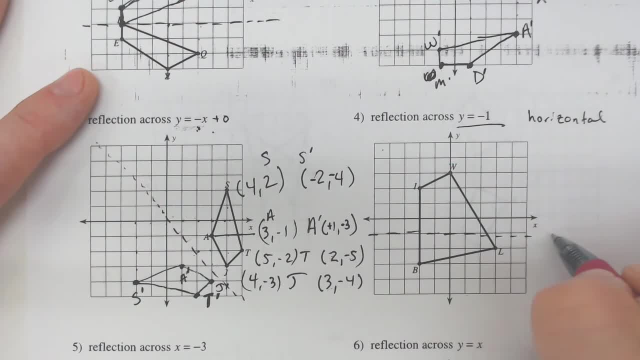 So Y equals negative 1 is right here. That horizontal line at Y equals negative 1.. And this time it's going to be a little bit of both, Like there's going to be some of the image that's below And some of the image that's above. 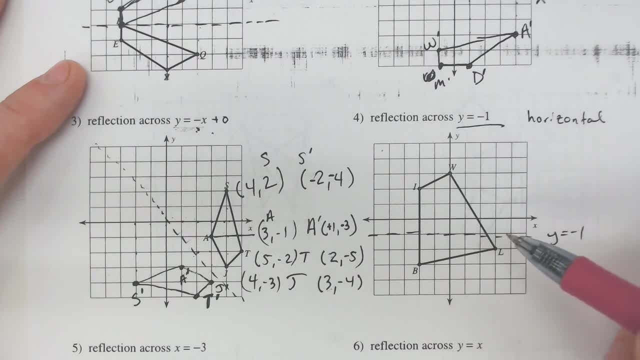 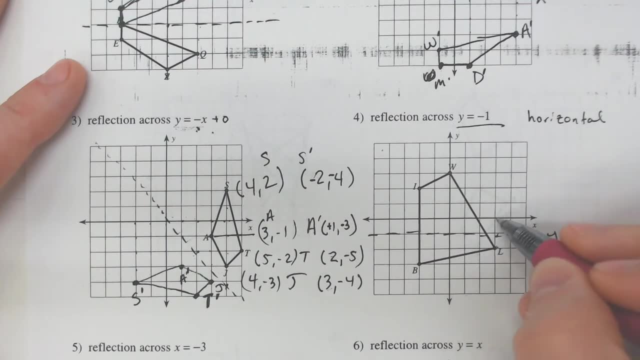 So when we draw this reflected image, It's going to actually kind of look like two things are overlapped. So I'm going to start with the bottom points. We would go up by 1.. So my L prime is going to be up by 1 up here. 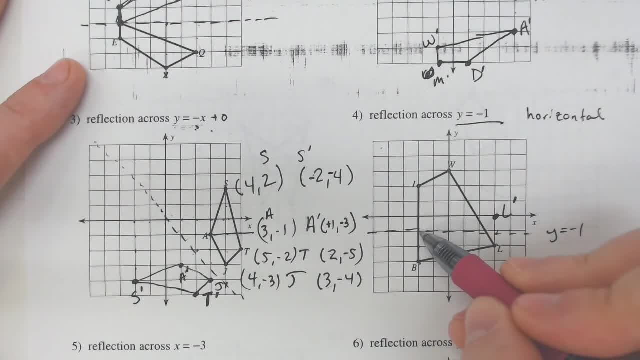 My B prime I would go up by 2.. So I got to go up by 2 more And it would be right here for B prime, My I- I went down by 1,, 2, 3.. I got to go down by 1,, 2,, 3 more for I prime. 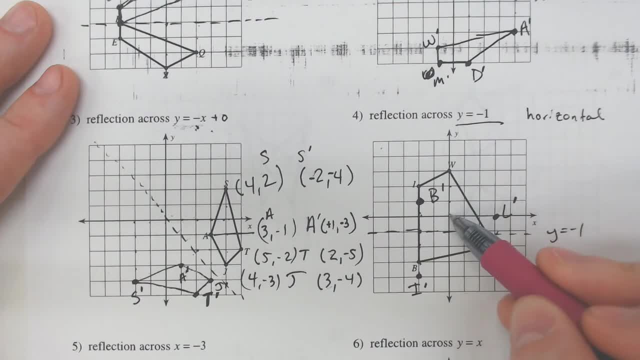 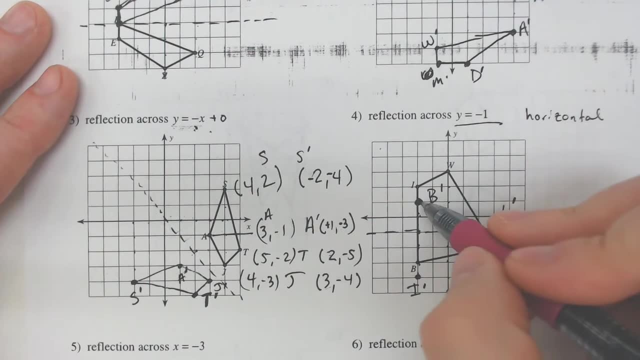 W went down by 1,, 2,, 3, 4.. I got to go down by 1,, 2,, 3, 4 for that W prime. I'm going to draw this one like with a dotted line. 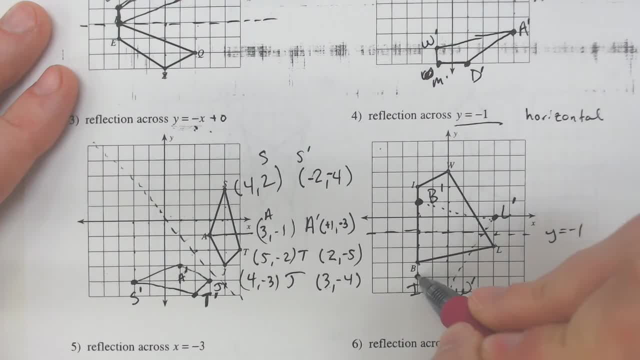 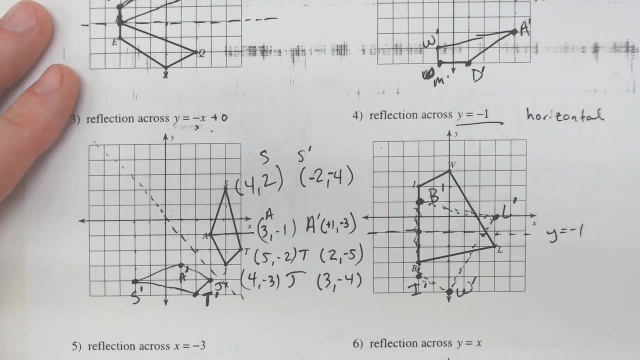 Just so that we can kind of see the original and the new shape a little bit more clearly, To see that, yes, they did reflect, But they kind of folded on to each other even more so. But that would be how you would do those. 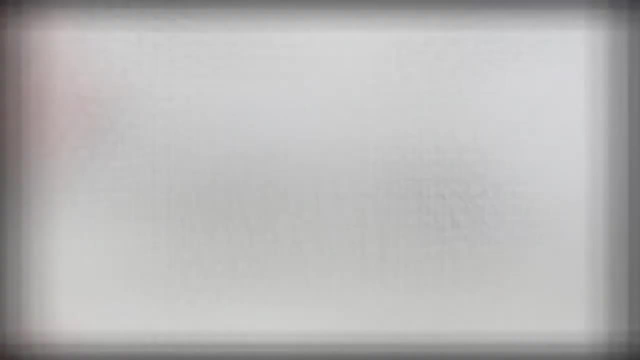 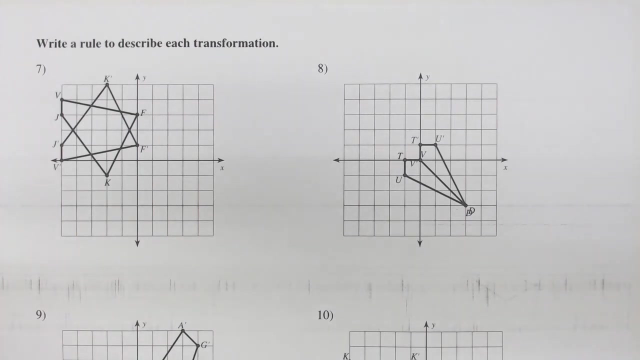 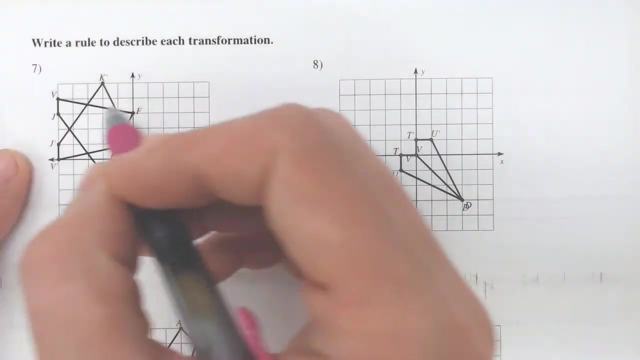 Now the next thing that we're going to be doing is going to be figuring out what is the line of reflection. So how did it reflect? And we have to draw where it was flipped over a mirror image of, So that one requires a little bit of just visualization. 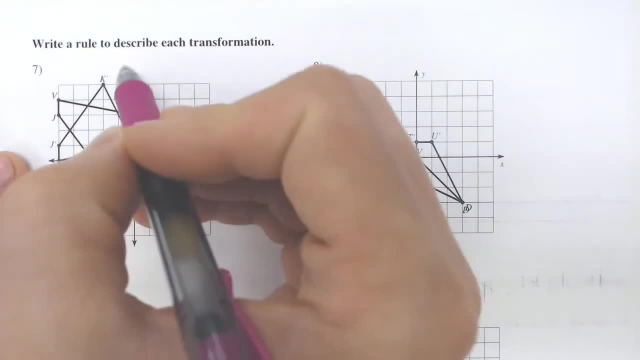 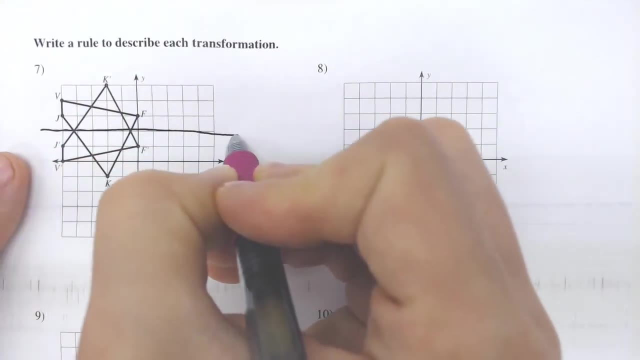 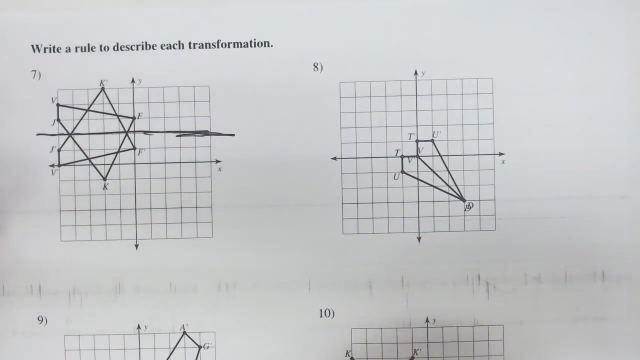 To see: well, did we draw the line here? If we drew that line there, would it actually fold on to itself, Or would it be here in the middle of that image? And I just drew the line of reflection because if I folded it over that line, 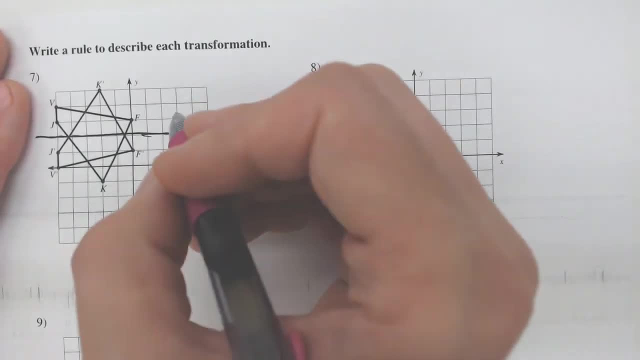 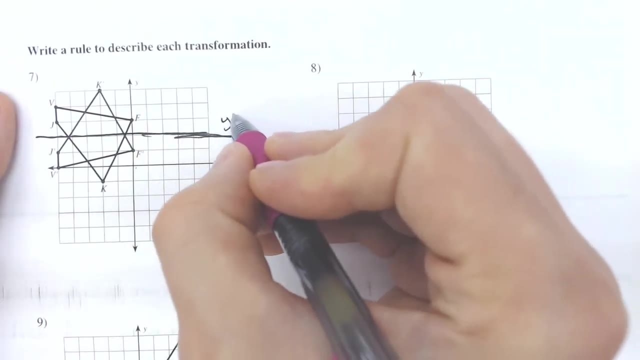 These two things would be able to fold on to each other. So what is that line that I just drew? Well, it's a horizontal line up at 1, 2 for the Y value. Horizontal lines are Y equals, The Y equals 2.. 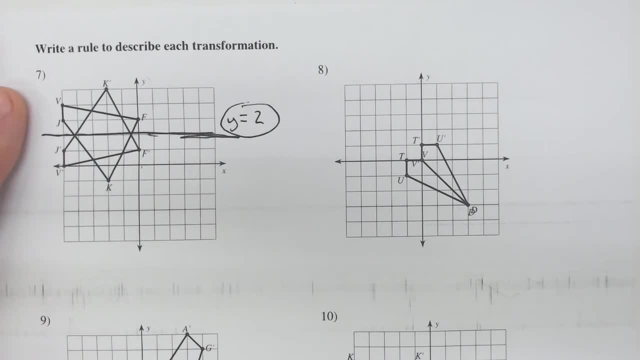 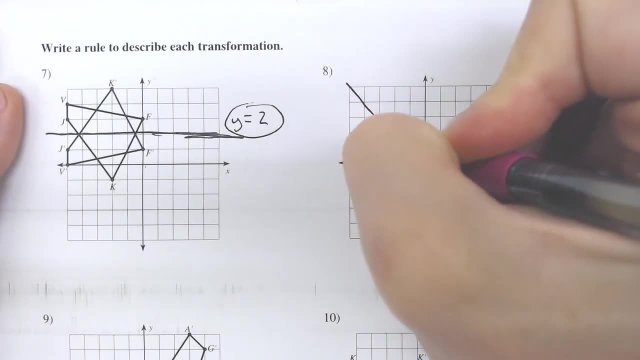 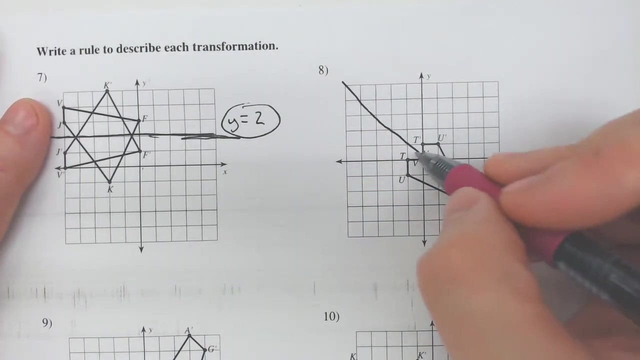 Would be the line of reflection For number 8.. The line of reflection is going to be diagonal, Which is no big deal. It's this diagonal line that I'm drawing right now. So what is this? diagonal line with a slope of negative 1 and a Y intercept of 0. 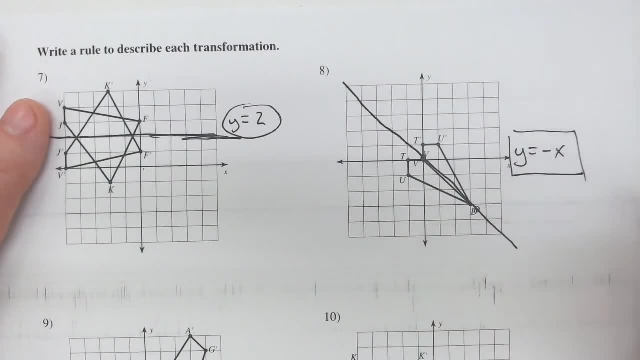 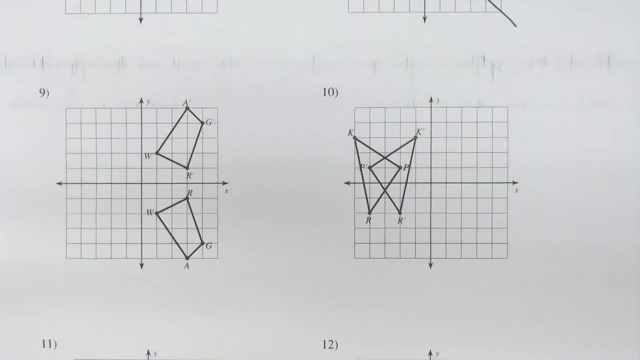 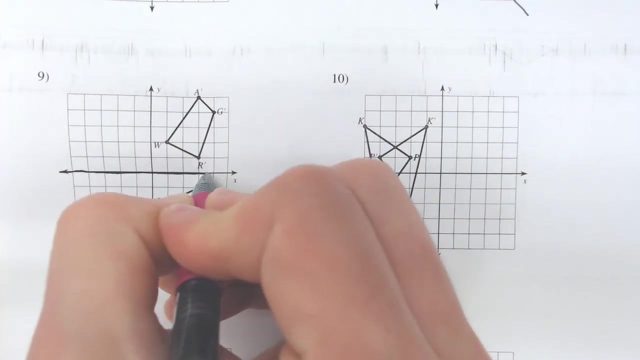 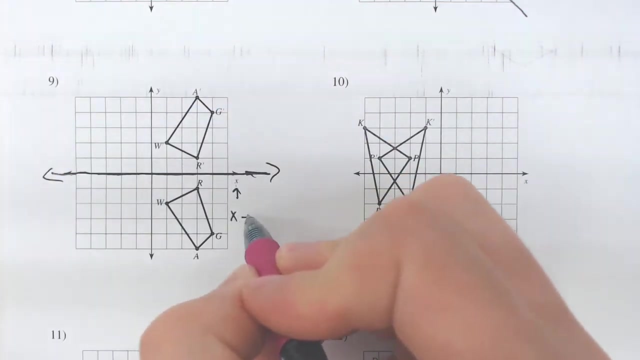 Well, that is, Y equals negative X. Diagonal lines are going to be the Y equals X or Y equals negative X. The next two are going to be relatively simple to see. The middle of this, where it was reflected across, is right here. Well, that is going to be the X axis. 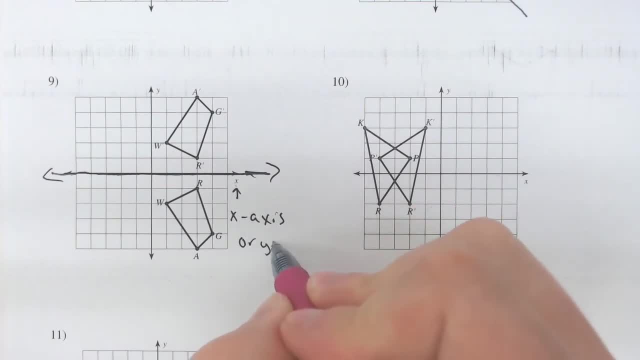 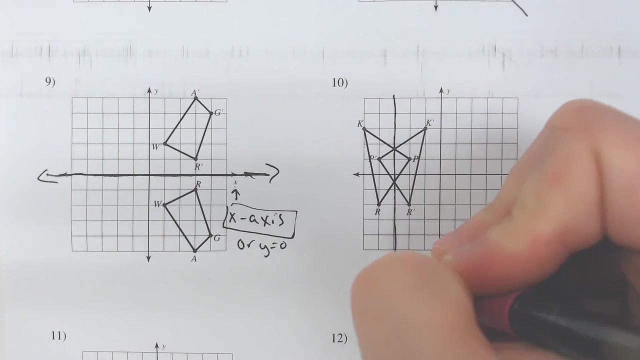 That's where we were going. You could have write: or equals Y, equals 0.. But most people would agree that it is the X axis that this got reflected across. This one Is actually reflected across this vertical line, So that vertical line. 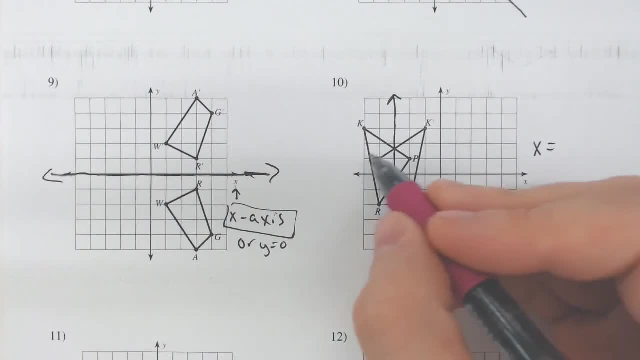 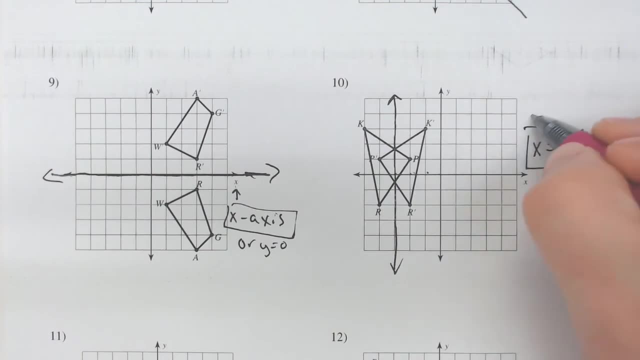 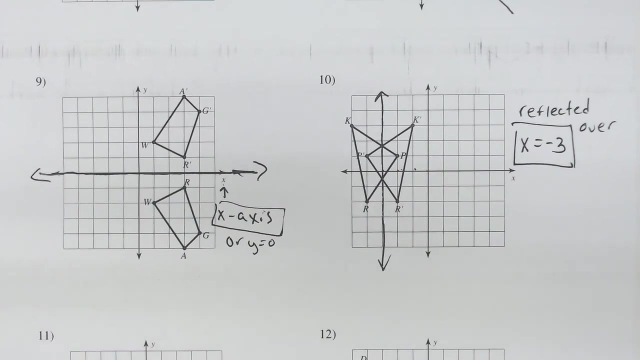 Is going to be an X equals And it's going to be X equals, whatever this vertical line is on, Which is 1,, 2, 3.. So this is going to be Reflected Over That: X equals negative 3..